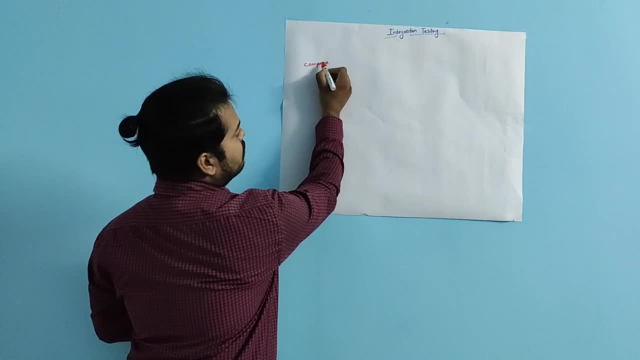 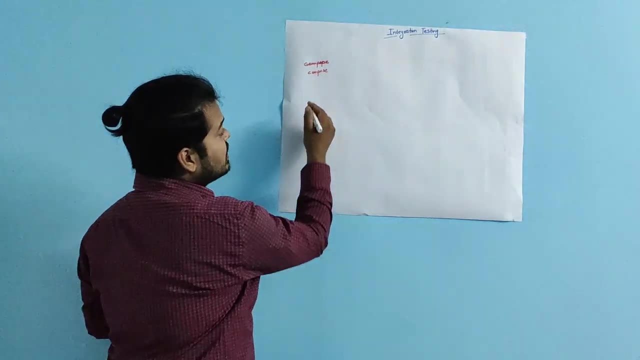 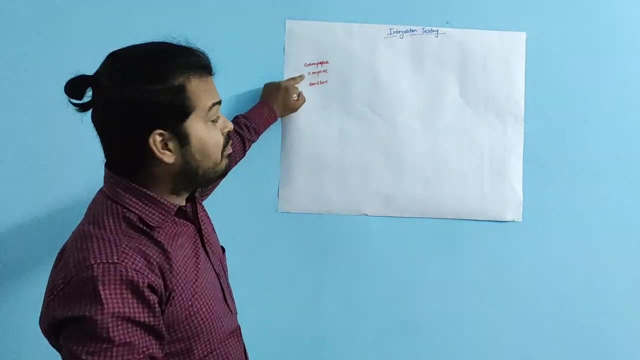 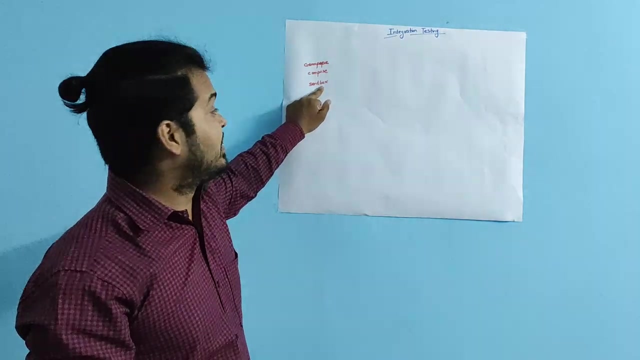 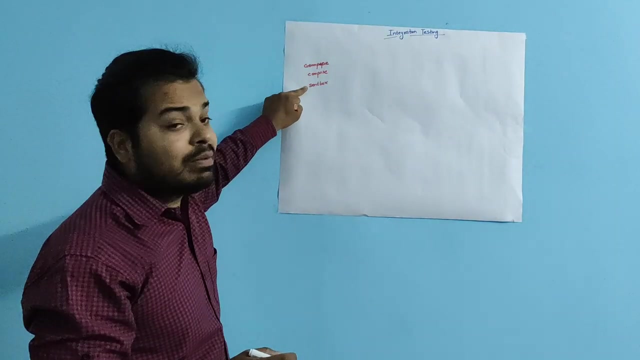 One is compose a mail And one more is send box. So you have sent a message from compose mail and you are checking the same mail is present in the send box or not. That is called as integration between the two modules. Your compose a mail is one module, Your send box is another module. 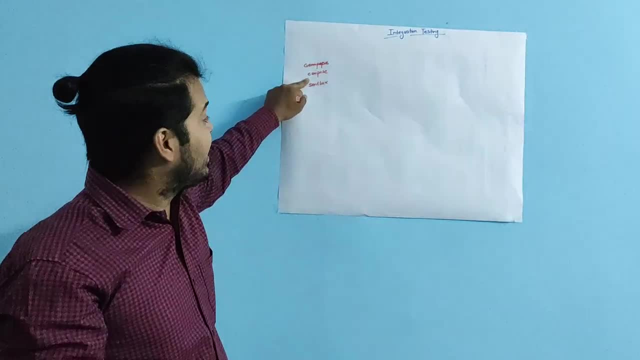 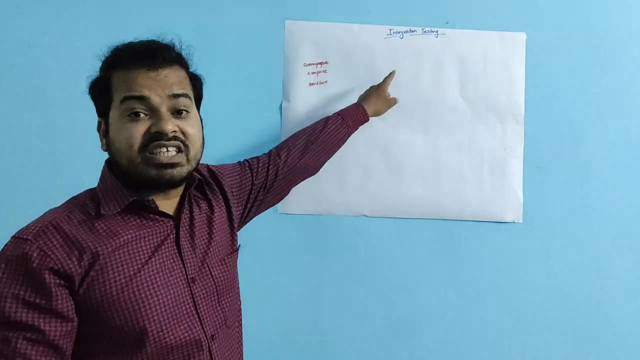 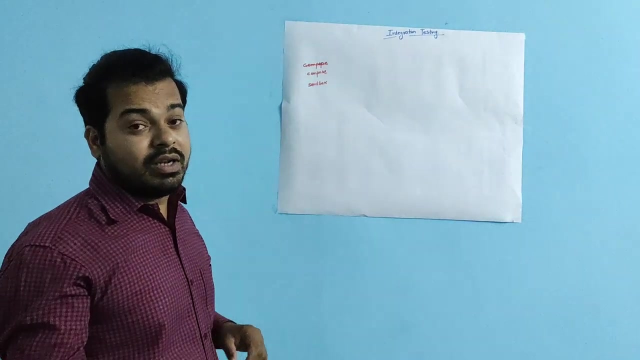 You have sent a message from composing it and you are checking it in the send box. That is called as integration between the two modules. Integration testing can be performed Between two modules or more than two modules. Let's take one more example of performing integration testing. 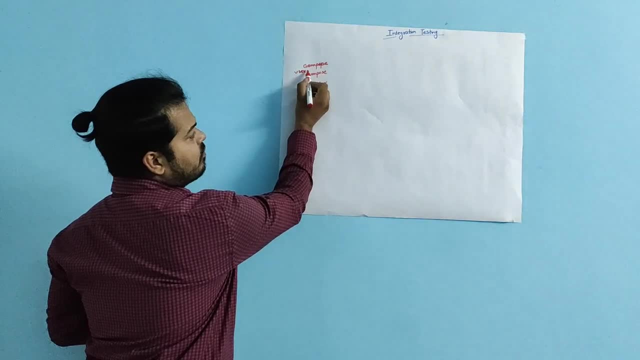 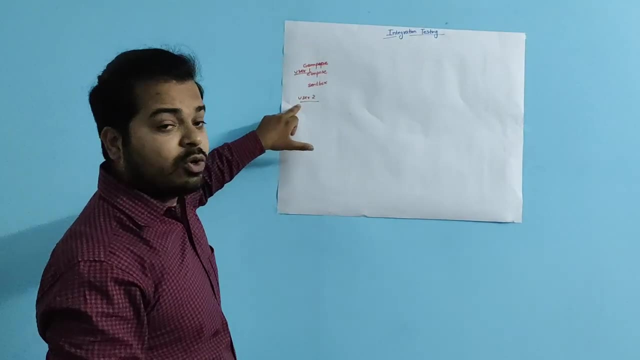 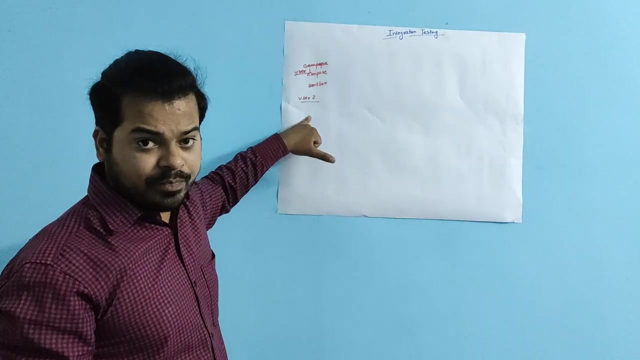 Suppose you have, this is user 1 profile and this is user 2 profile with their user name and password. User 2 is with their user name and password. Now you have created a compose mail. You have sent it to the user 2.. 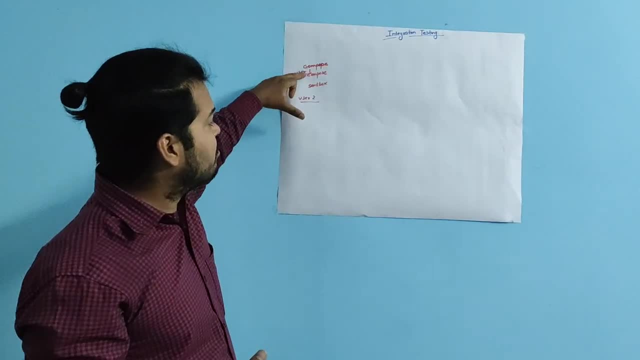 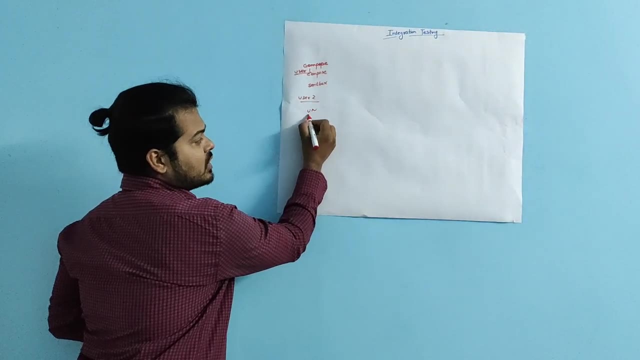 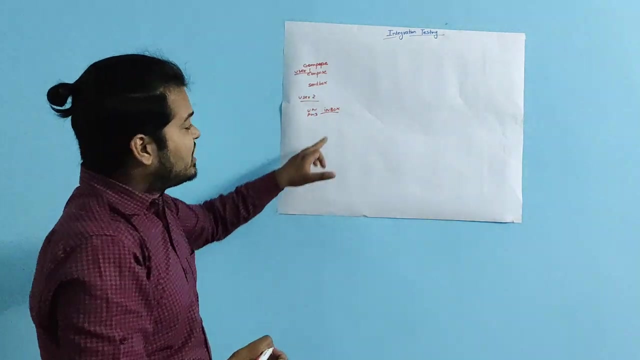 Now you have tested the integration between compose and send. Now I will log in to the user 2 credential by entering his user name and password and I am checking his inbox. I am checking his inbox. I am checking whether that mail which he has compose and send it to the user 2 is present in this inbox or not. 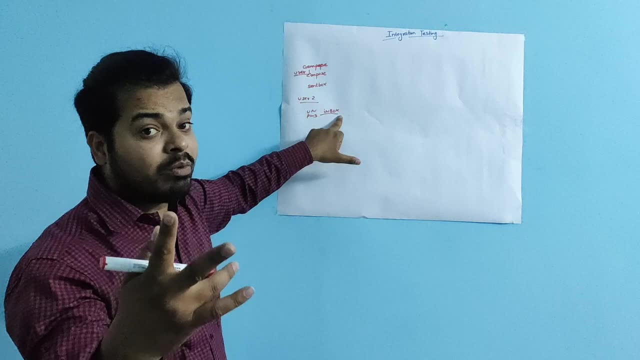 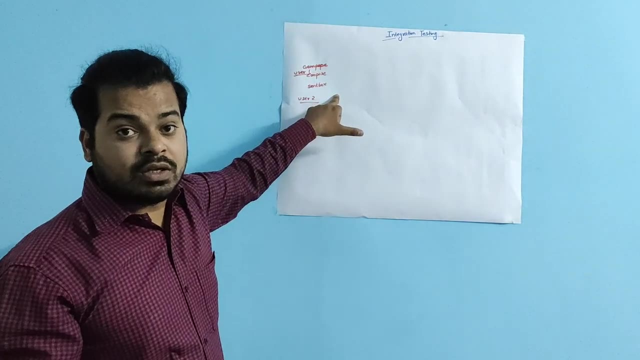 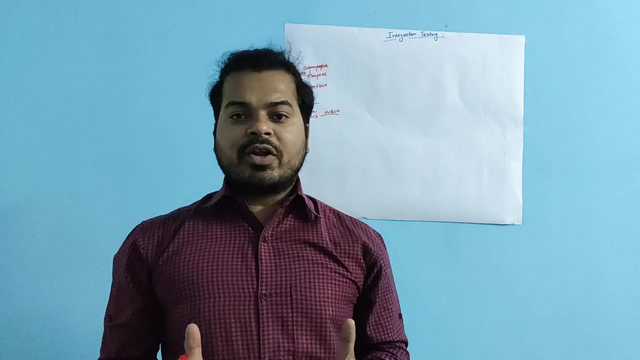 I am verifying the integration between the two modules. One is in the inbox of user 2.. One is from the user 1 compose. This is called as integration testing. I hope this is understandable by you guys. Now we are going to discuss the types of integration testing. 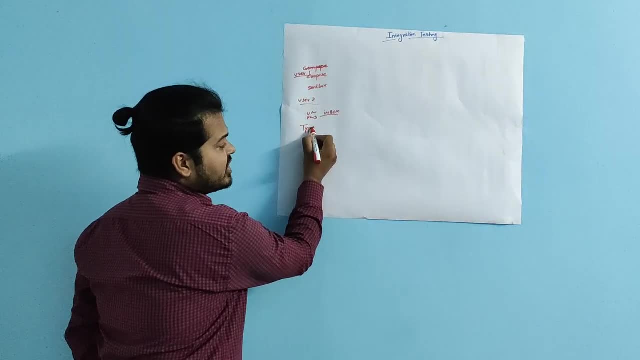 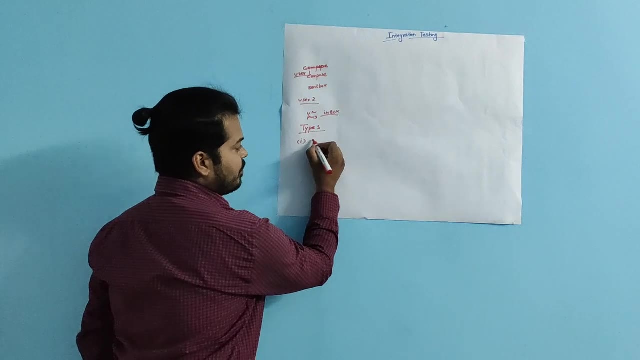 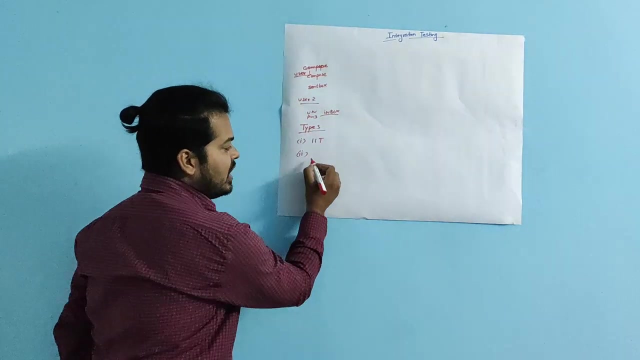 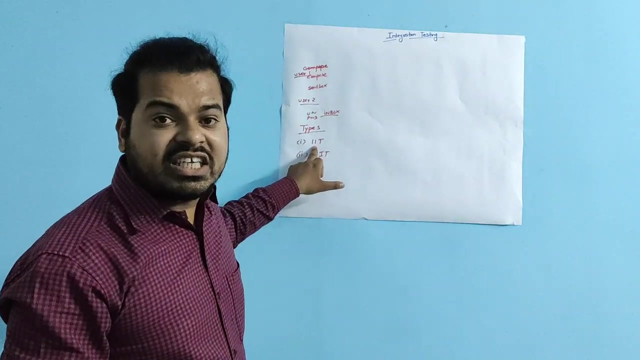 So the types of integration testing are: First is called as incremental integration testing, Incremental integration testing. And the second type of integration testing is called as non-incremental testing. Non-incremental testing is testing. Now, what do you mean by incremental integration, Incremental integration testing? says that incrementally adding the modules and testing the data flow between the modules. that is called as integration testing. Suppose there is an application with only module A. Now you are adding module B and checking the integration between them. That is called an incremental integration testing: Incrementally adding the modules and testing the data flow. between them. that is called as incremental integration testing. I hope it is clear. In incremental integration testing there are two types. The first is called as top down incremental integration testing And the second is called as top down incremental integration testing, And the third is called 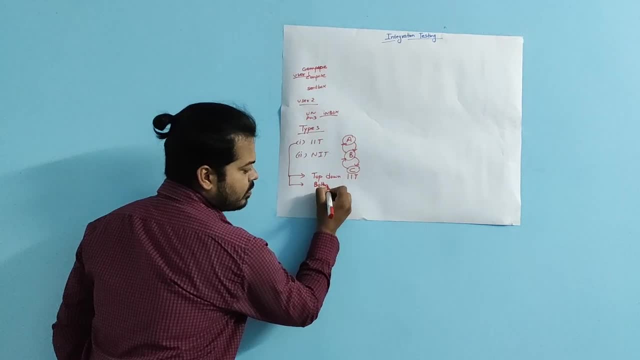 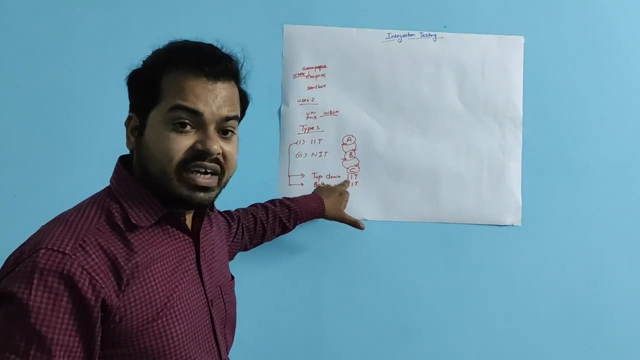 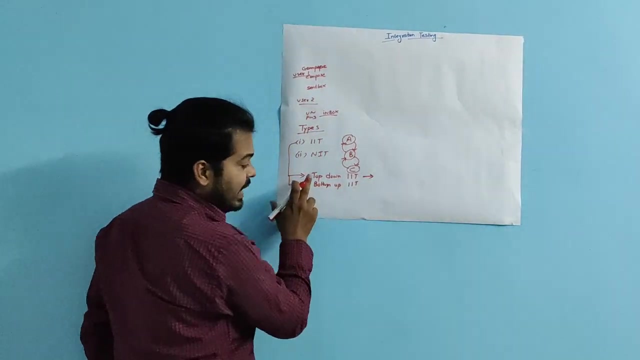 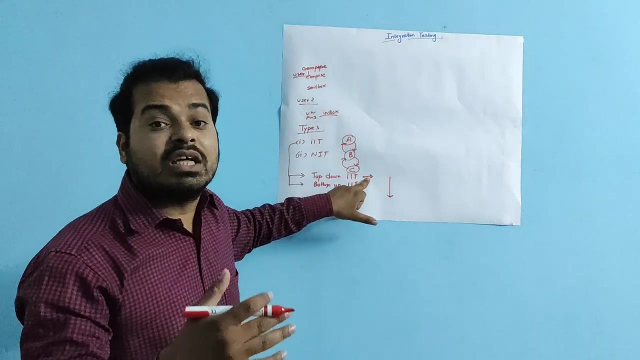 top down- incremental integration testing, And the fourth is called as top down incremental integration testing And the fifth is called as top down- incremental integration testing. Now, what do you mean by top down incremental integration testing? top down, as the name suggests, top down Incrementally, adding the modules and testing the data flow between. 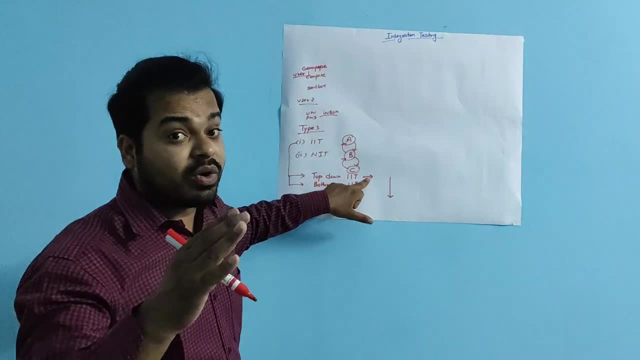 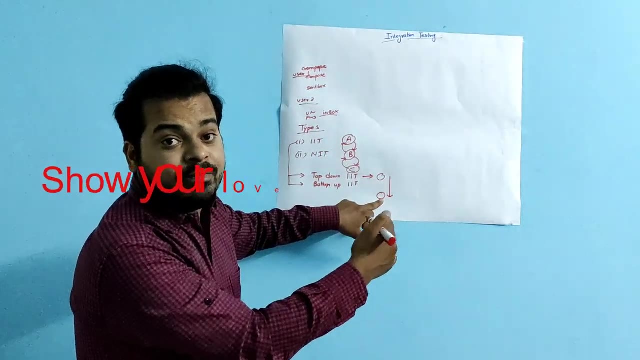 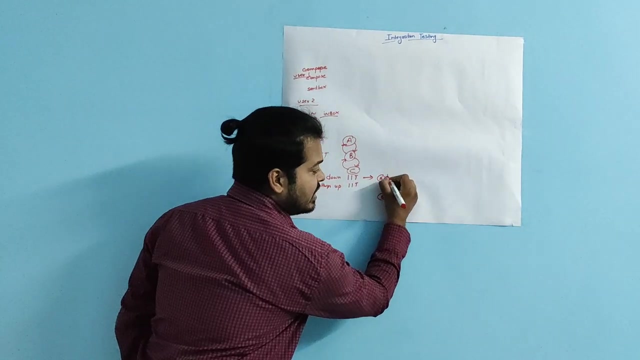 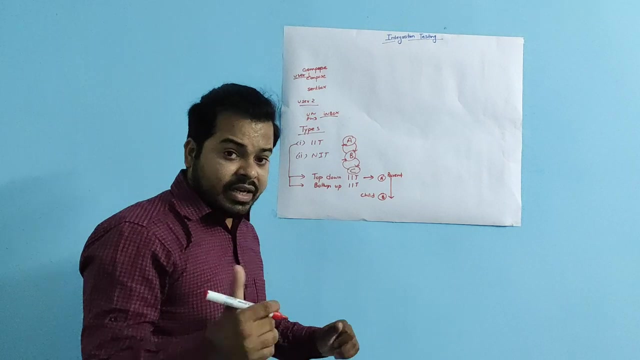 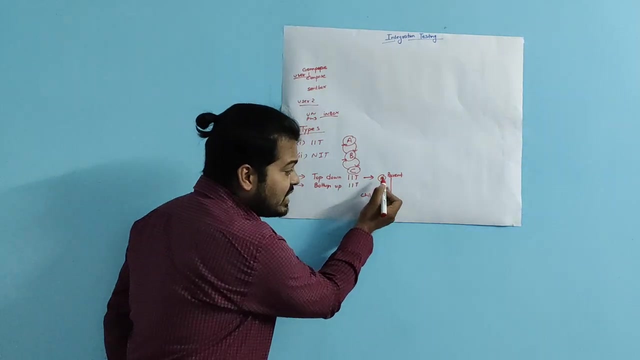 testing the data flow between them and ensure the modules that we are adding. is the child of the previous module. that means this is my one module, a module. this is my second module. that is B. this is parent module. this is my child module. now, top-down incremental integration testing says that incrementally adding. 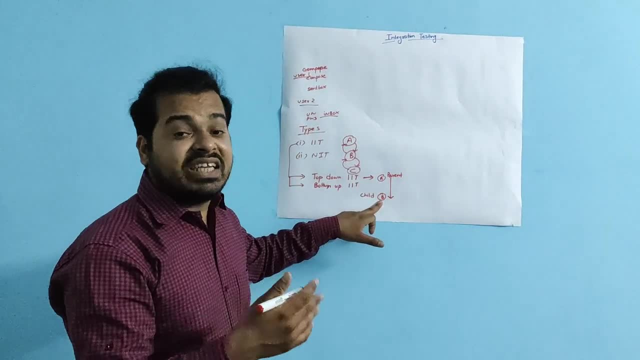 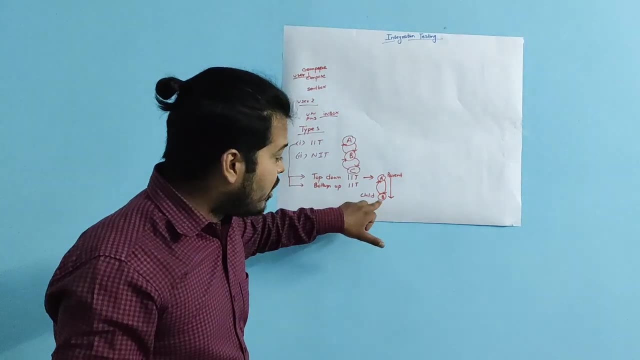 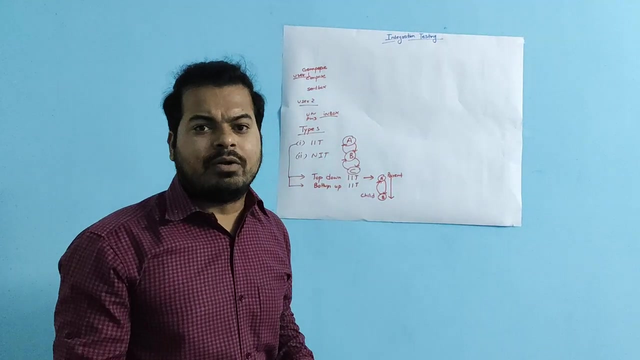 the modules, that is B, and testing the data flow between them. you are testing the data flow between A and B and ensure the modules you are adding is the child of the previous module. now, what do you mean by child and the parent module? guys, I want to give you example. let's take an example of 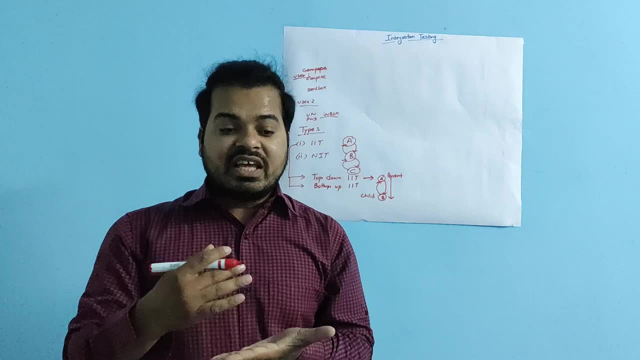 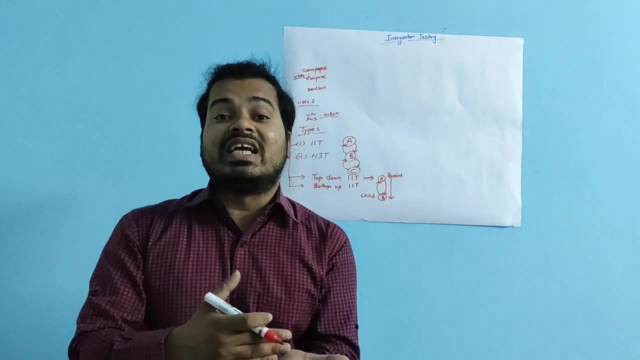 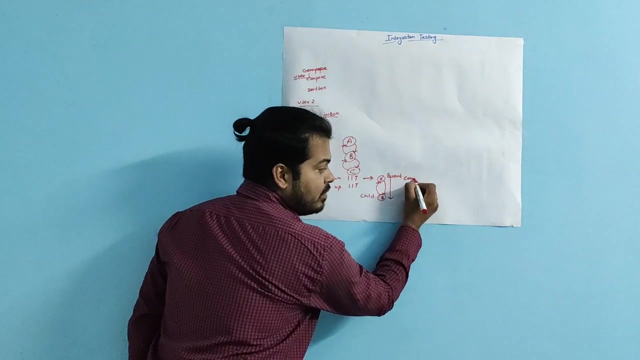 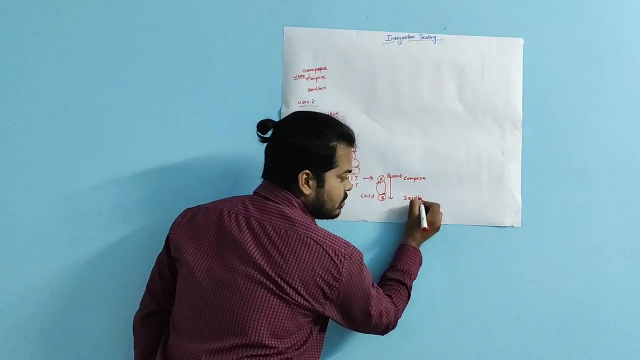 Gmail itself, where you are composing a mail. if you are sending the mail, then only will come to the sent box, but if there is no compose, there won't be any send item. that means in this case: who is the parent module? my compose mail is my parent module. who is the child module? my sent box. 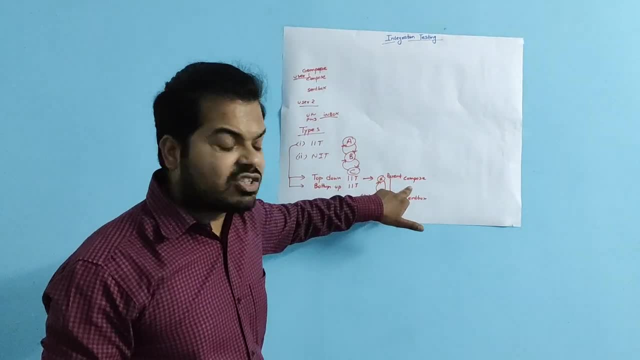 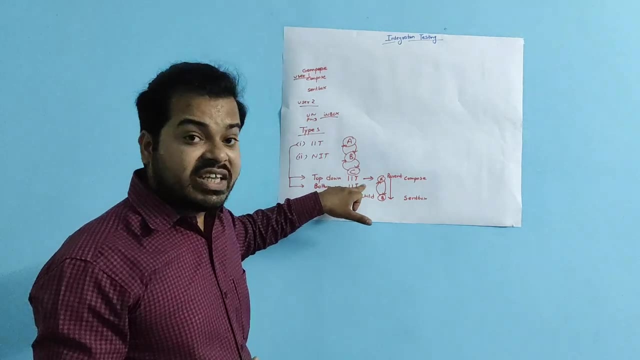 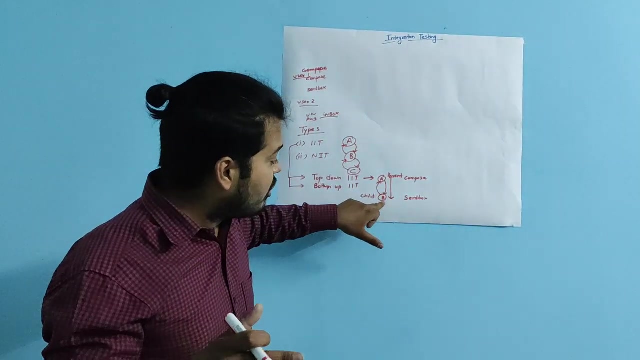 the reason we are telling compose as a parent module, because if compose is soup there, sent box won't be there. that is why we are telling top-down incremental integration testing mean incrementally adding the modules, testing the data flow between them and ensure the module which we are adding is the child of the. previous module that is called as top-down incremental integration testing. I hope it is clear now. the second type of incremental integration testing is called as bottom of incremental integration testing since, as the name suggests, it is bottom up, so from bottom your going bottom up. incremental integration testing says that incrementally adding. 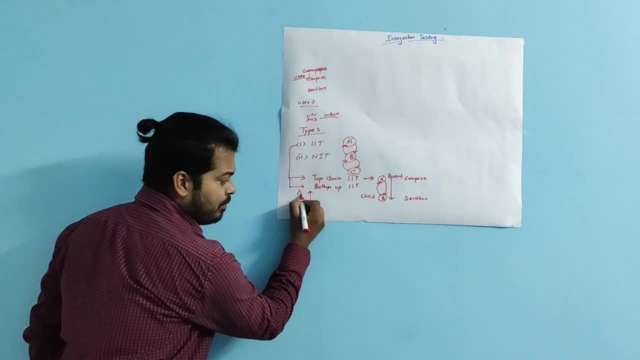 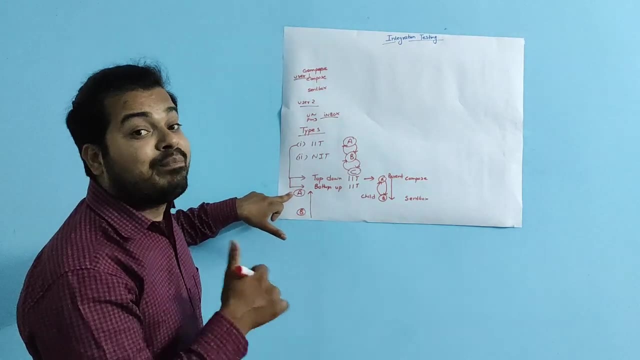 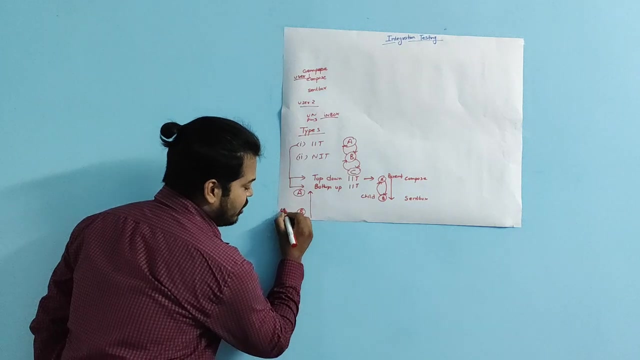 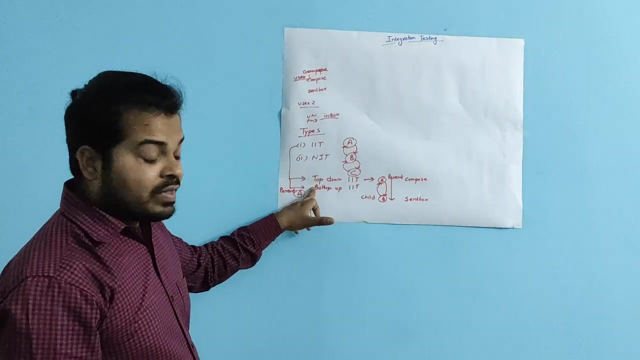 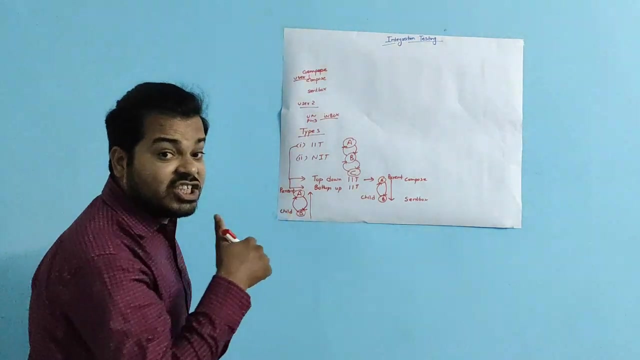 the modules, testing that data for between them and ensure that the module which you are adding is the parent of the previous model. that means if this is my, this is my child module. this is my parent module, since it is bottom up. I am incrementally adding the modules and testing the data flow between them and ensuring the module. 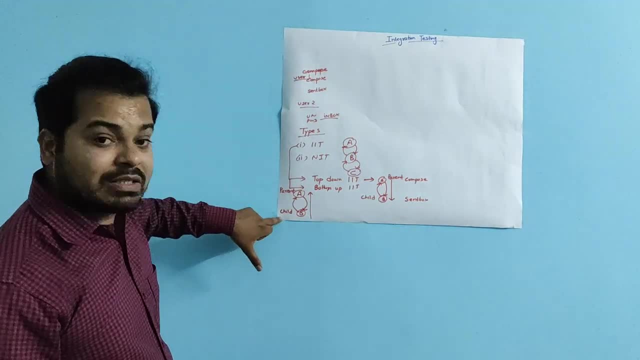 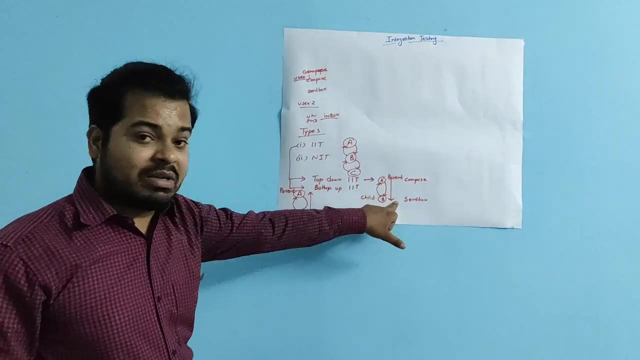 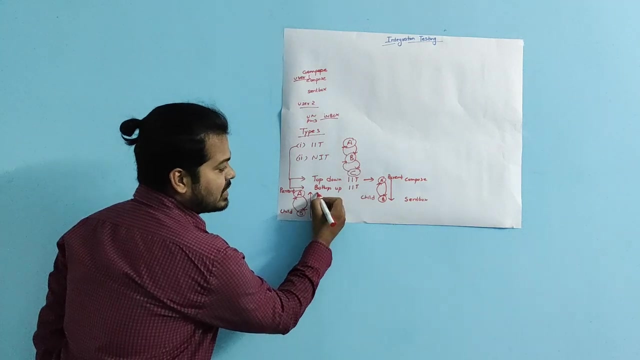 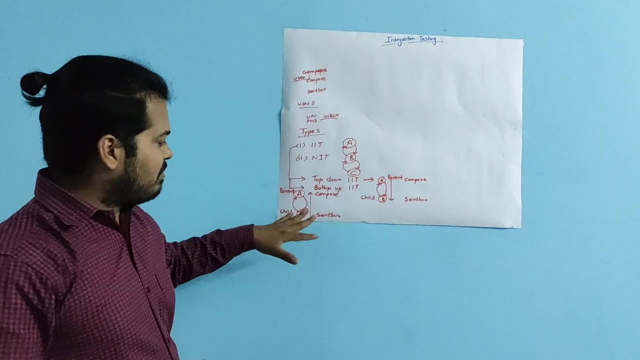 that I have added is the parent of my previous module. that is called as bottom-up incremental integration testing. I'm going to take the same example. suppose my B is my sent box, my parent is my compose module. see you, never just reversing it. so in bottom-up incremental integration testing. 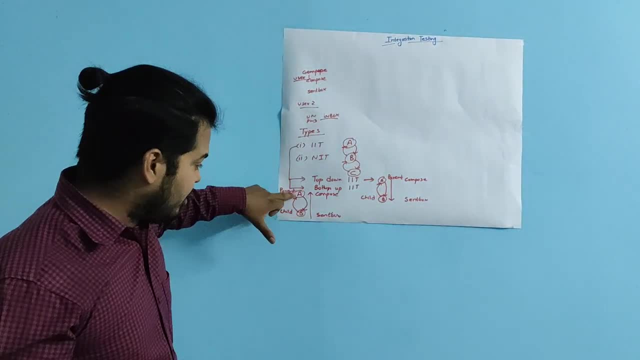 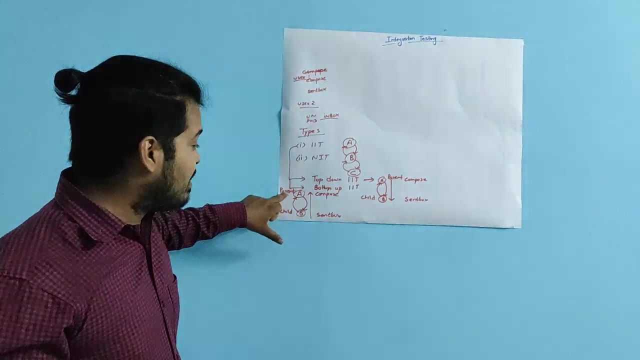 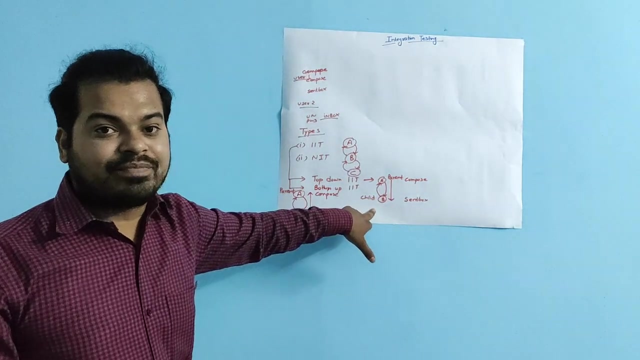 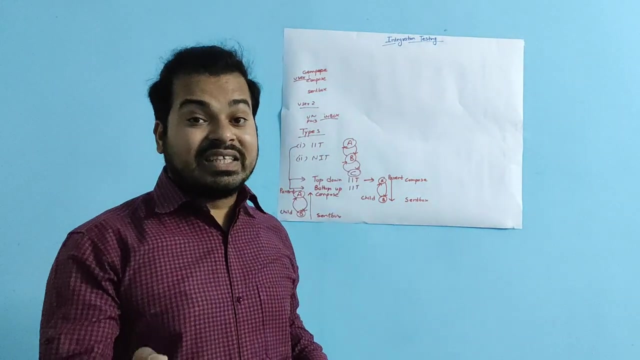 you are incrementally adding the module and testing the data flow between them and ensuring the module which is added is the parent of the previous module. that is called as bottom up, incremental integration testing. I hope this clear, guys. there is one interview question in this topic which any interviewer can ask. that is: what do you mean by sandwich testing, guys? always. 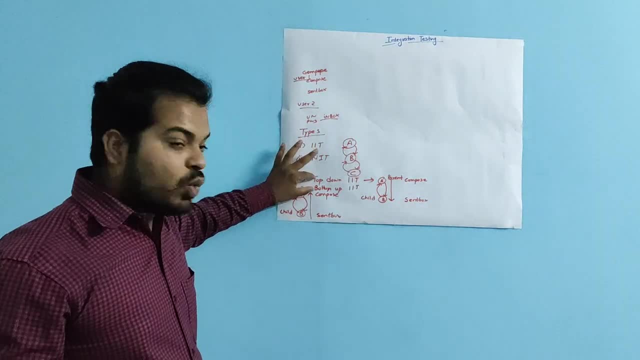 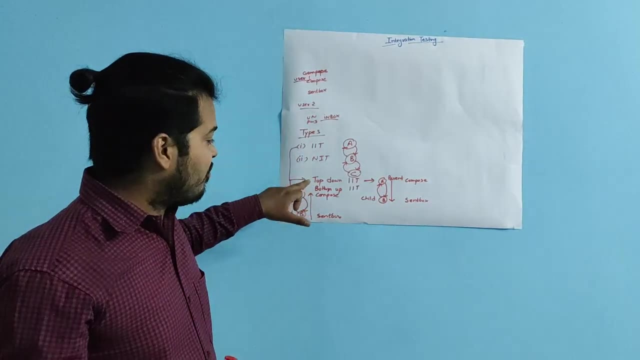 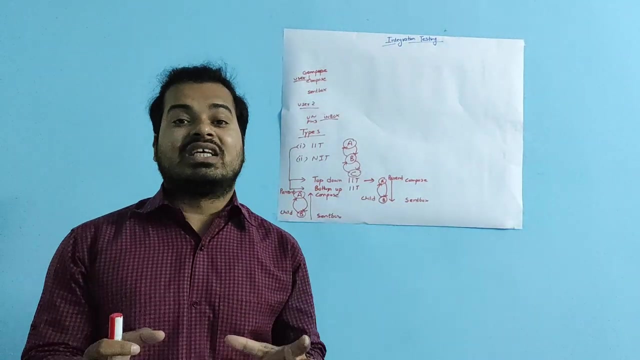 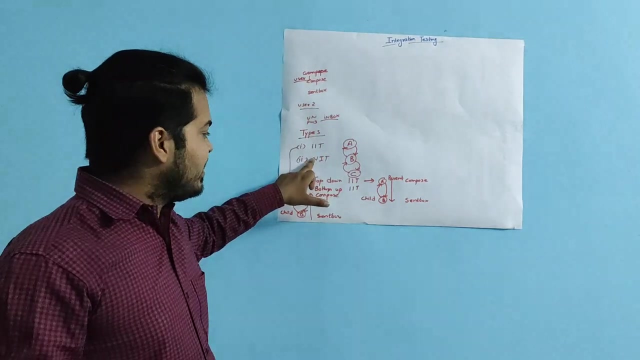 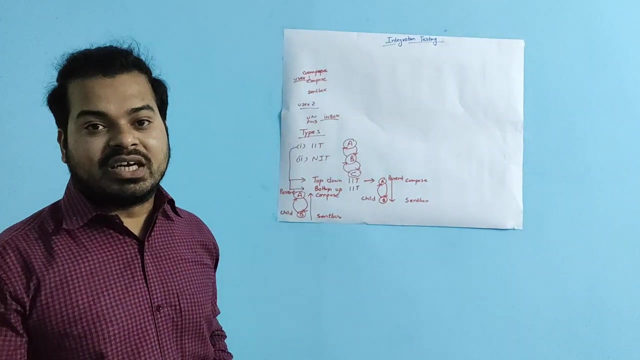 remember the combination of my. this two is called as sandwich testing. now, what is the definition? the combination of top down incremental integration testing and bottom up incremental integration testing. it is called as sandwich testing. coming to second type of integration testing that is known incremental integration testing, which is also called as big band method. 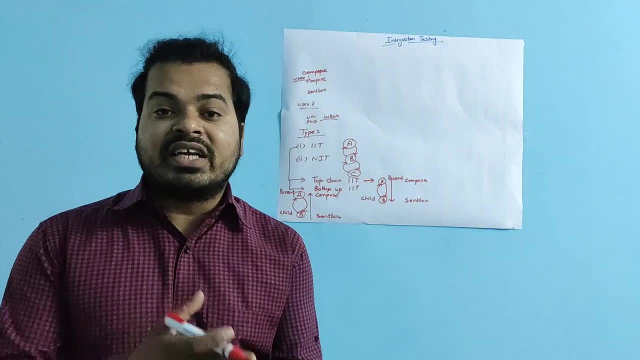 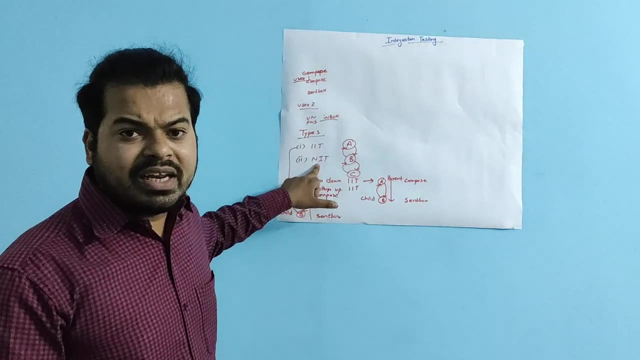 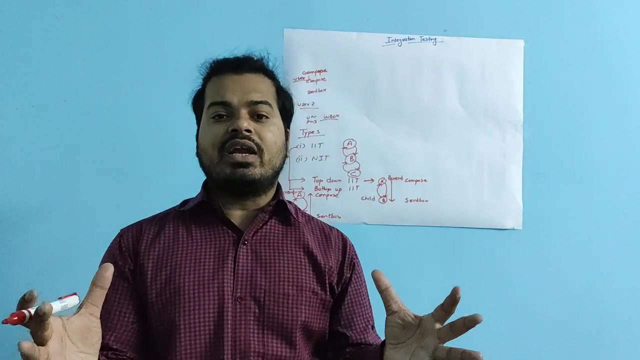 an interview. they can ask you either to explain non incremental integration testing on, as they have done, ask you directly to explain big bank method. so what do you mean by non-incremental integration testing? in non-incremental integration testing, you are adding all the modules in a single shot. 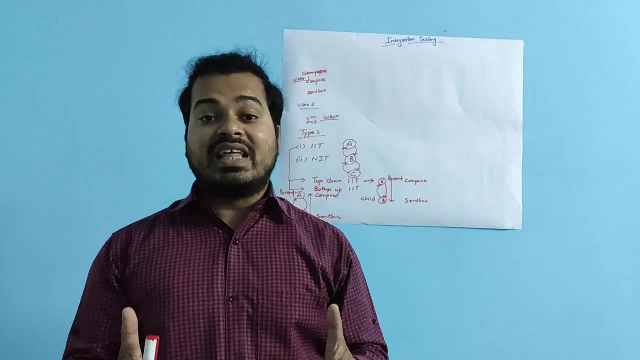 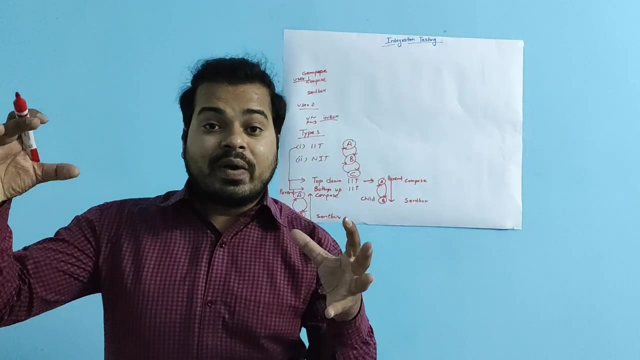 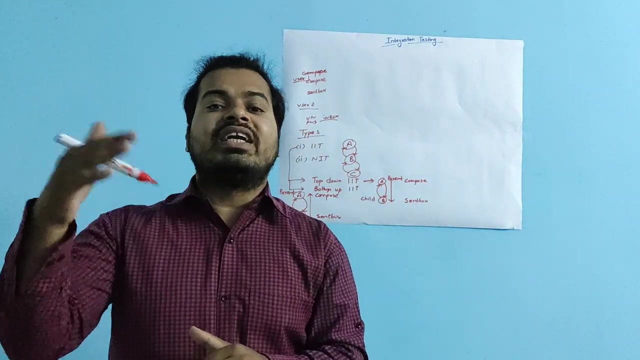 and you are trying to test the data flow between them. that is called as non-incremental testing. in non-incremental testing, you are adding all the modules, whichever present in the application, in a single shot. and now you are trying to, you are trying to do the integration testing between 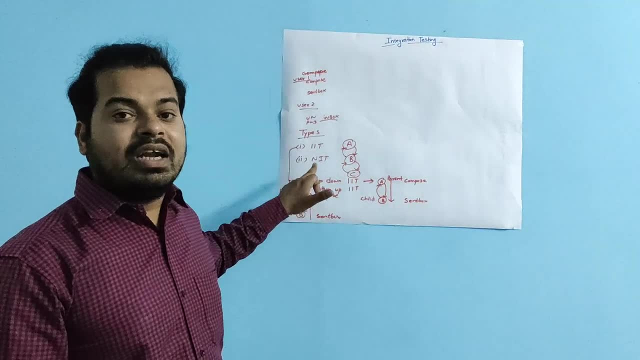 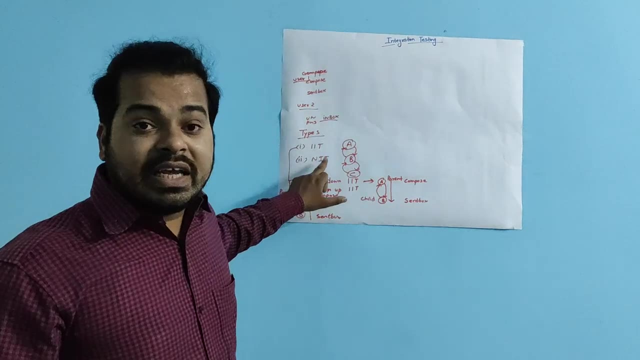 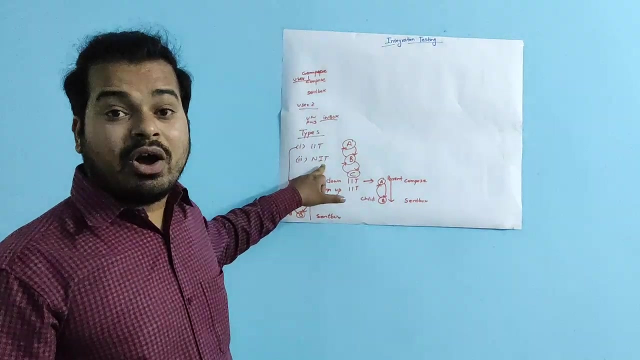 the models that is called as non-incremental testing. whenever we don't know the parent and the child module, we go for non-incremental testing. i hope it is clear. now the question arises: what are the drawbacks of choosing a non-incremental testing? so the first drawback of choosing a 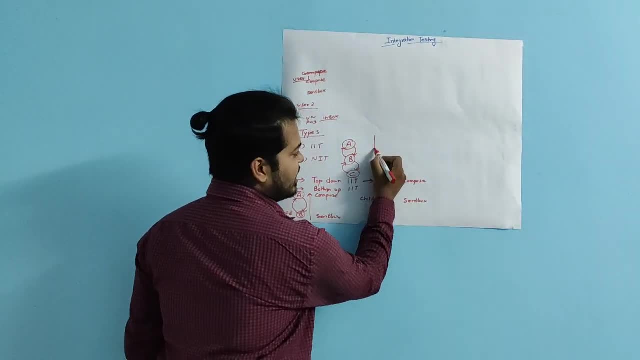 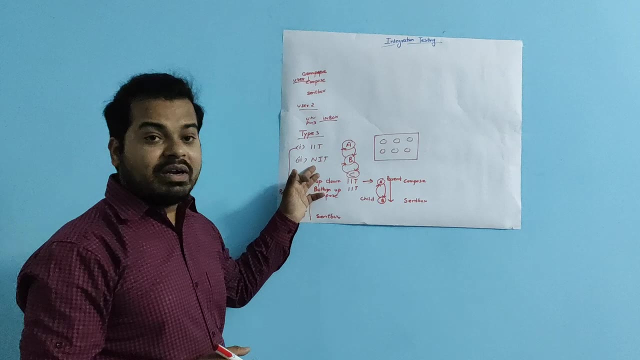 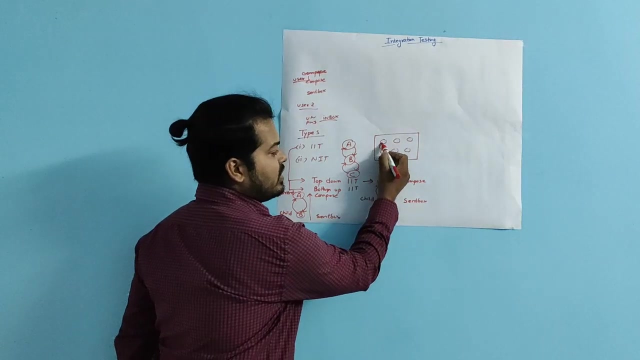 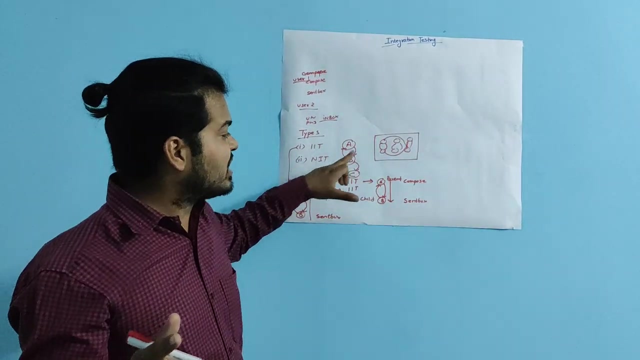 non-incremental testing is suppose this is our application, in which there are many modules in it. what non-incremental integration testing says? that? or adding all the modules in a single shot and testing the data flow between them. so the first drawback of non-incremental testing is we might miss to test the data flow between. 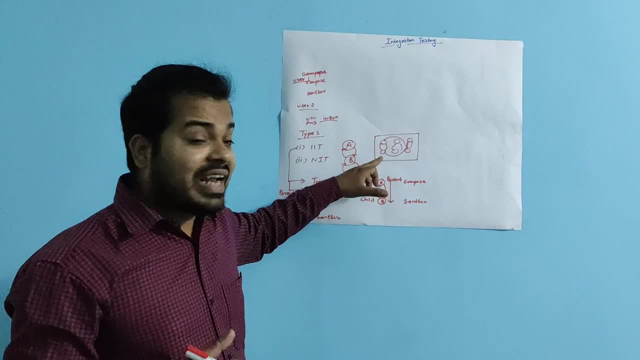 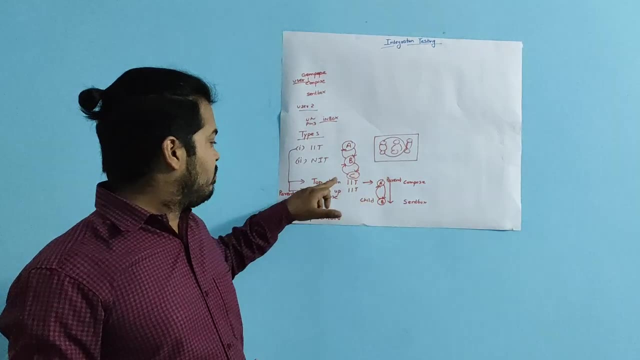 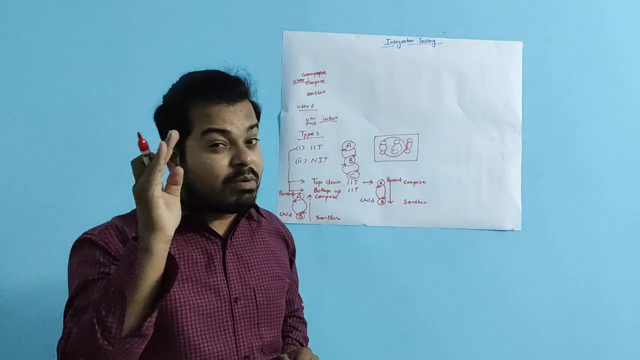 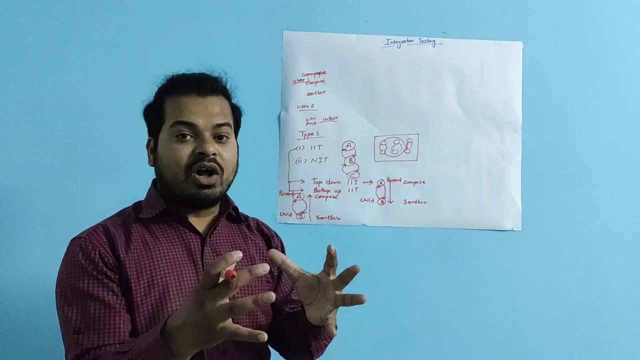 some of the modules. second, we might end up testing the same module- integration testing- again and again and while doing non-incremental testing, if, if you are finding any defects, we won't be able to understand the root cause of the defect, since there there are many modules in it and we have added the all the modules in a single shot. if we are finding any. 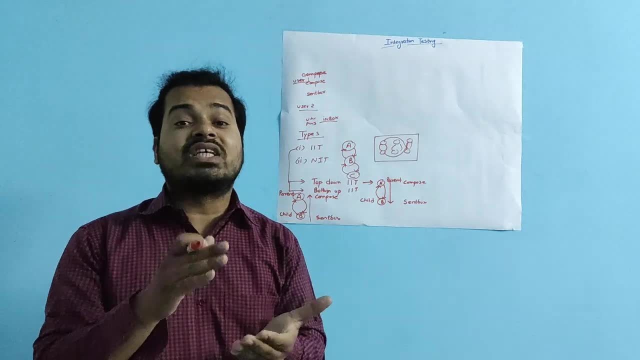 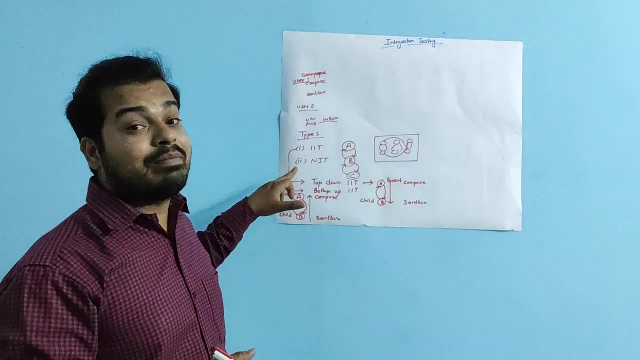 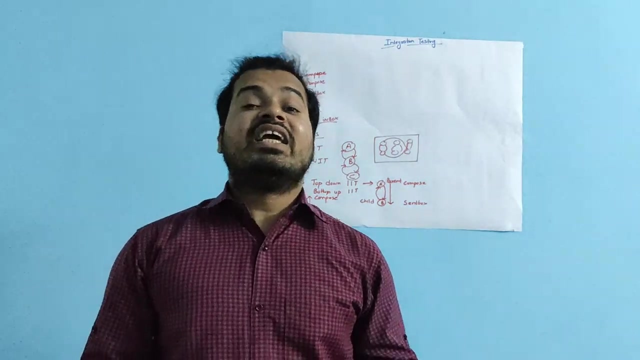 bug or defect, we won't be able to understand what is the root cause of it. that is called as non-incremental testing. these three are mainly called as the drawbacks of non-incremental testing. i hope this video is useful to you guys. make sure that you like this video. subscribe to my channel. 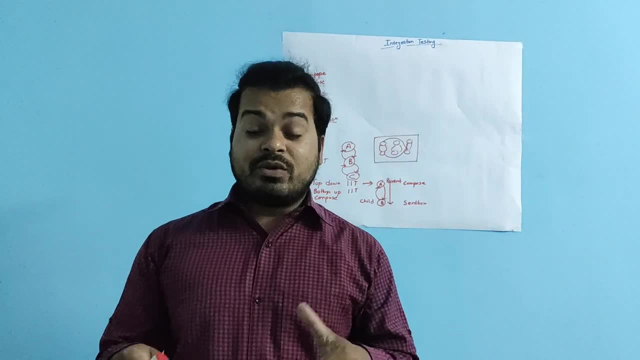 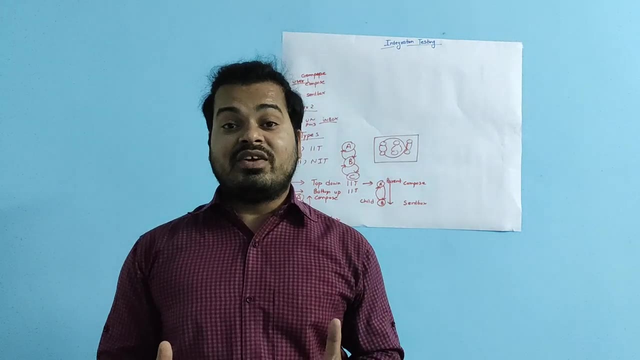 if you have any doubt in this related to this video, make sure that you list out in the comment section i will be answering. like this video. subscribe to my channel and never miss any video from software testing by mkd.